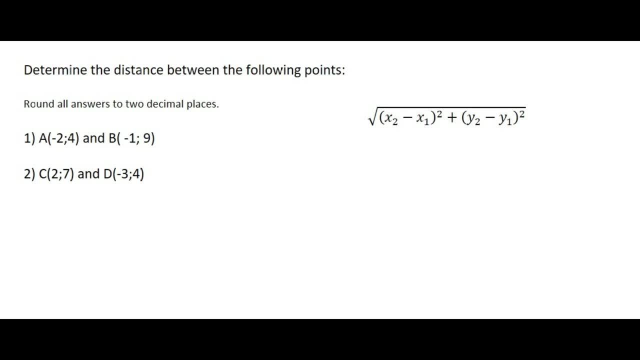 So you choose. let's say you just choose A or B as your point number two. So I'm just going to do it like that. It really doesn't matter. I promise you, no matter which way you do it, you will get the same answer. 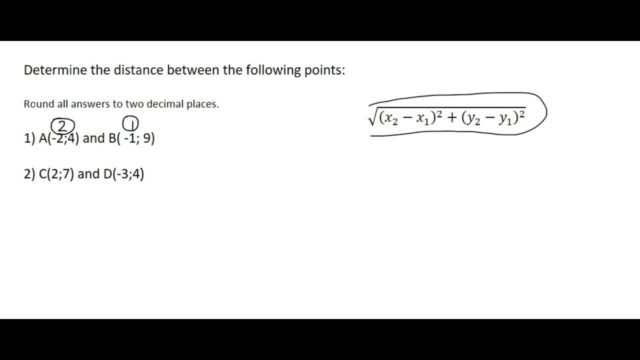 So now we just use this formula. Remember, this is the distance formula which is actually doing Pythagoras. Many people don't know that It's actually just doing Pythagoras. I know I've mentioned that a lot, but it just fascinates me that that formula is doing Pythagoras for us. 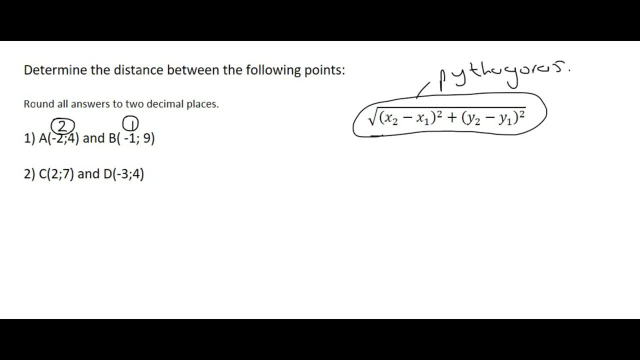 But many people think that it's just a brand new formula. but actually no. So let's go fill in the formula. So it says that there's a square root, and then we can do this like this, And then I'm going to fill in everything. 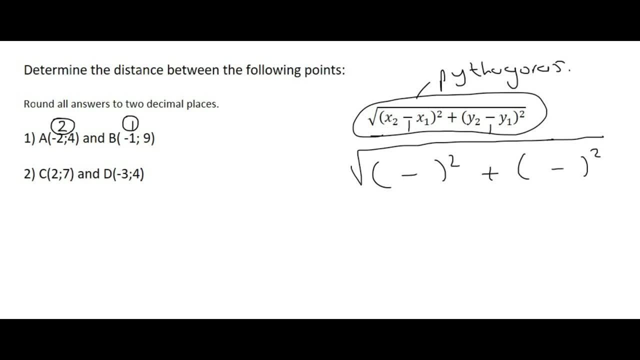 It should be there. so there's a minus, There's a minus over there. And then it says I must take the x value of point number two. So point number two is A. Now which of them is the x value? Is it the minus two or the four? 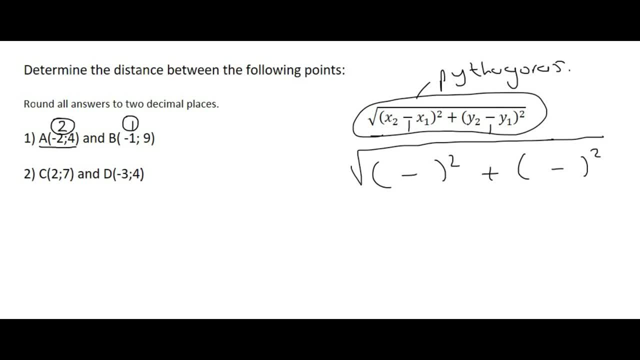 Well, the x is always the first one, so that's always going to be the minus two, just like x is first in the alphabet, So that's going to be a minus two. Then it says I must use the x value of point number one. 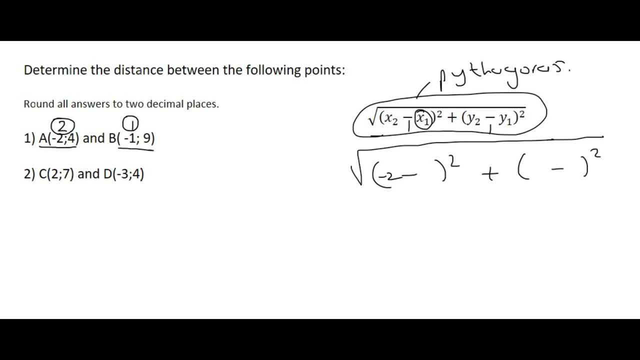 So I go to point number one, which is this one: Now, is the x value the minus one, or is it the nine? It's the minus one. Okay, Then the formula says I must use the y value. of point number two. 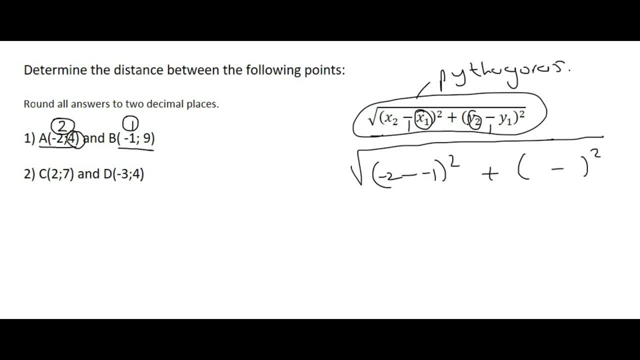 So point number two is A, So that's going to be the four. So I put a four over there, And then the y value of point number one is nine. You see, you literally just go plug everything in. Then what you do is you use your calculator. at this point. 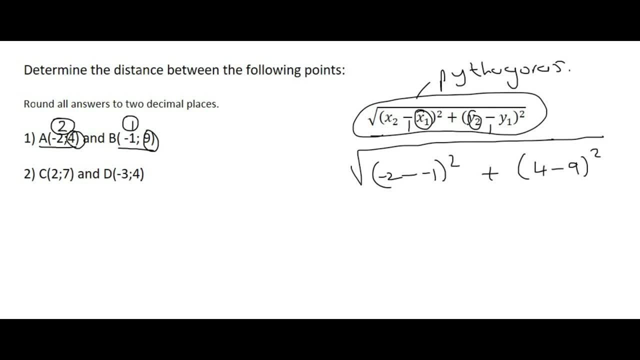 and you type it in exactly as you see it and the calculator will take care of all of the pluses and minuses and things like that, And that's going to give you the square. So if I'm at this point, I can't see the square. 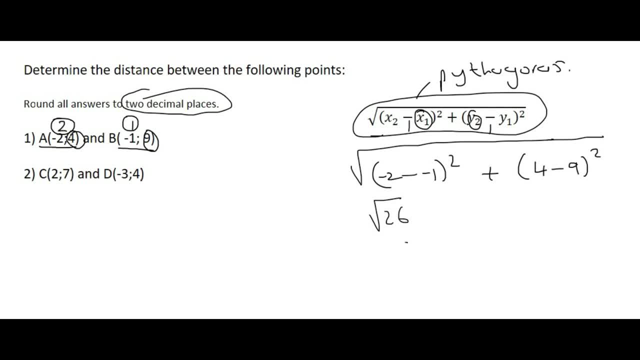 So I'm putting it in the square. So I put the four over there. So I'm going to use the formula to figure out that This is a minus one over there. So I'm going to put one over here. I'm going to put a four over there. 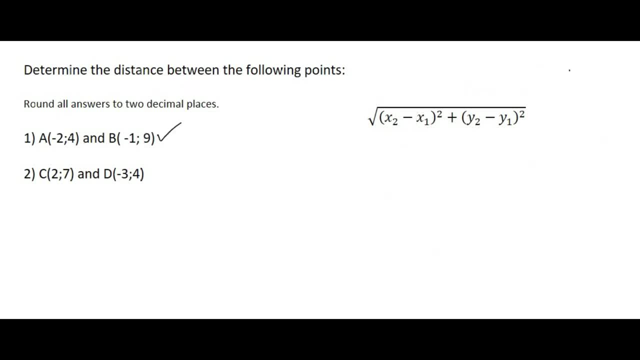 I'm going to use this formula to figure out that. I'm going to use both of the numbers. I'm going to use the formula to figure out the square root of 26.. But this question has asked us to do this to two decimal places.